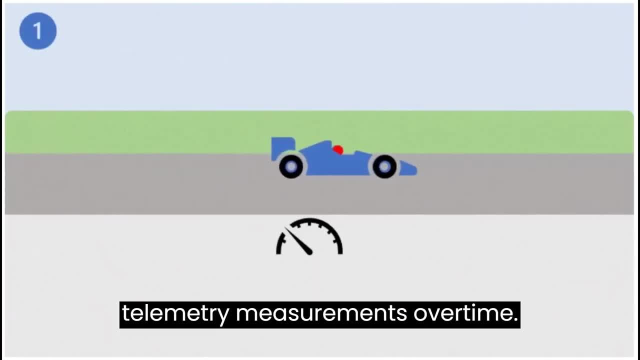 understand expected fluctuations in the telemetry model. If a measurement occurs outside of the normal expected range, the model reports an anomaly that can be used to alert the race engineer, to call the driver in for a pit stop to fix the issue before it forces retirement from the race. Next unit: what is computer vision? 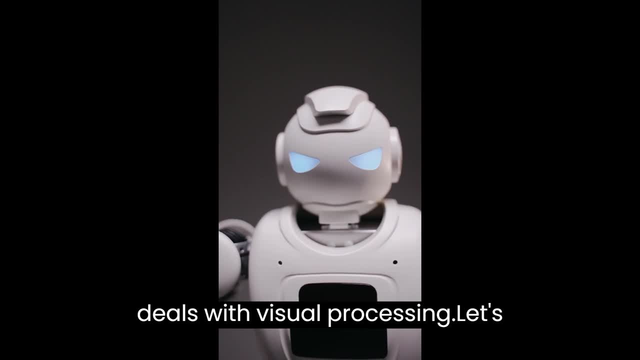 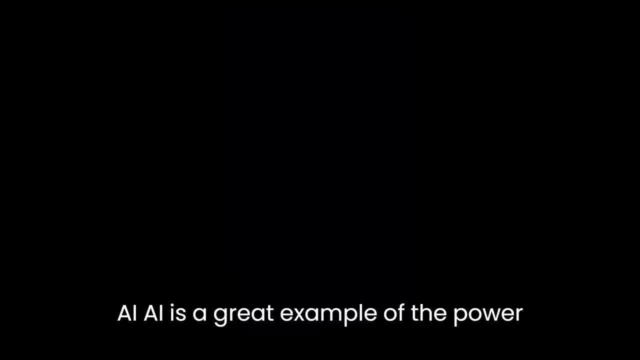 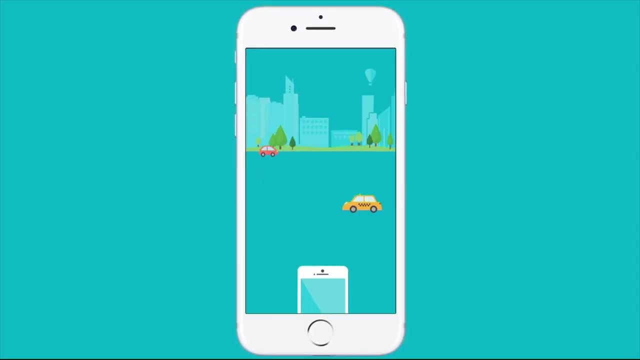 Computer vision is an area of AI that deals with visual processing. Let's explore some of the possibilities that computer vision brings. The Seeing AI app is a great example of the power of computer vision. Designed for the blind and low vision community, the Seeing AI app harnesses the power of AI to 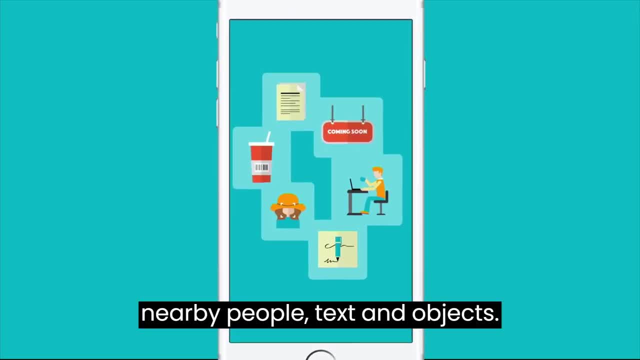 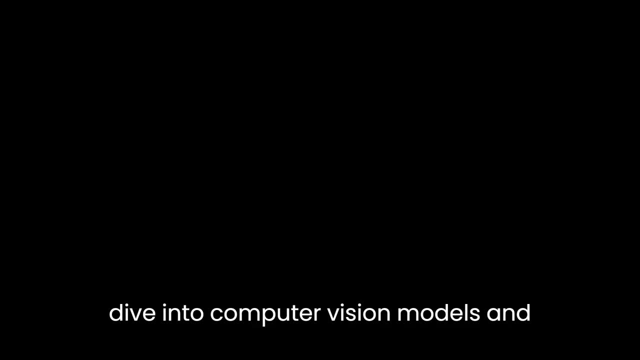 open up the visual world and describe nearby people, text and objects. I suggest you to check out their website, Seeing AI web page. Let's deep dive into computer vision models and capabilities. Number 1,: Image Classification. Image classification involves training a machine learning model to classify images based on their contents. 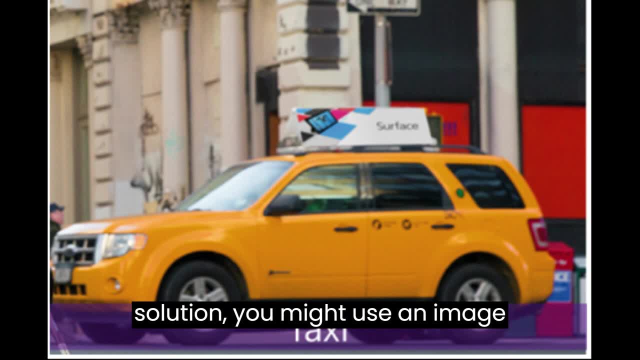 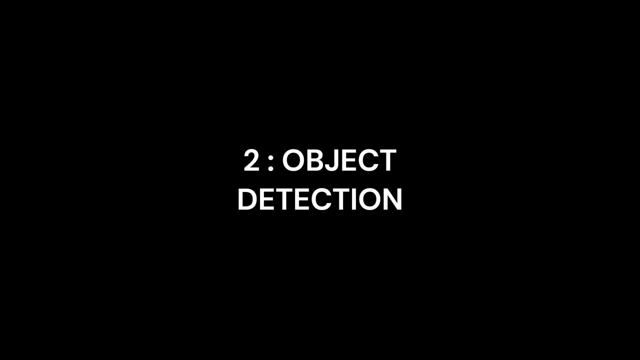 For example, in a traffic monitoring solution, you might use an image classification model to classify images based on the type of vehicle they contain, such as taxis, buses, cyclists and so on. Number 2, Object Detection. Object detection- machine learning models are. 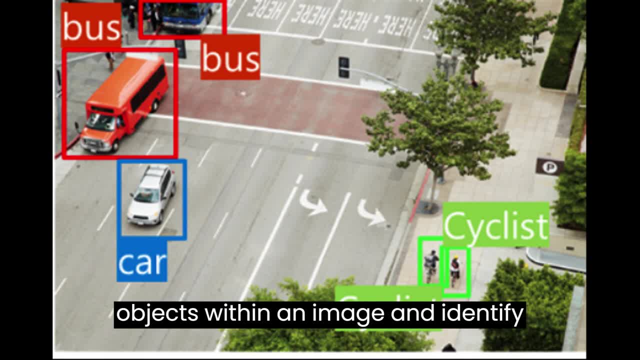 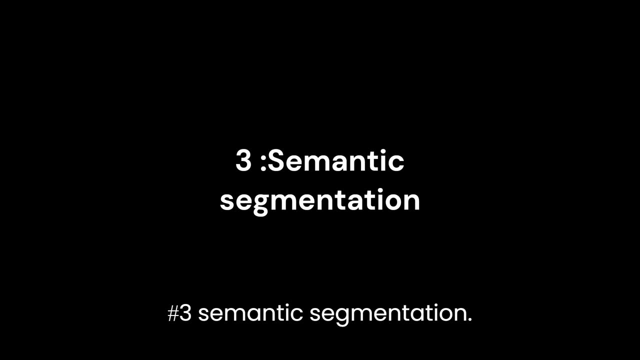 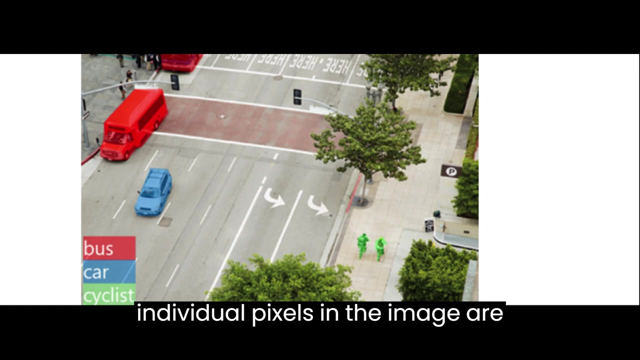 trained to classify individual objects within an image and identify their location. with a bounding box, For example, a traffic monitoring solution might use object detection to identify the location of different classes of vehicle. Number 3, Semantic Segmentation. Semantic segmentation is an advanced machine learning technique in which individual pixels in the image are classified according to. 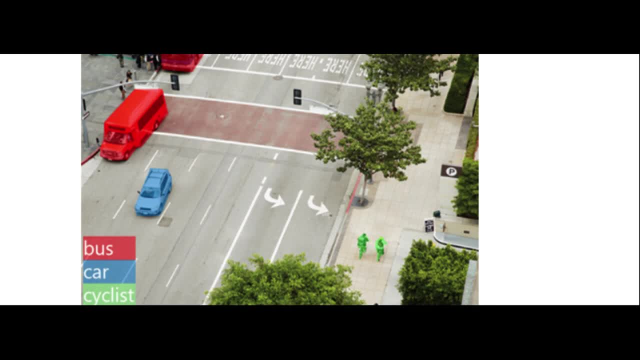 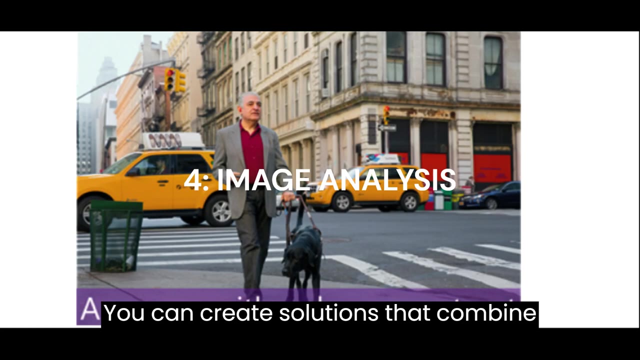 the object to which they belong. For example, a traffic monitoring solution might overlay traffic images with mask layers to highlight different vehicles using specific colors. Number 4, Image Analysis. You can create solutions that combine machine learning models with advanced image analysis techniques to extract information. 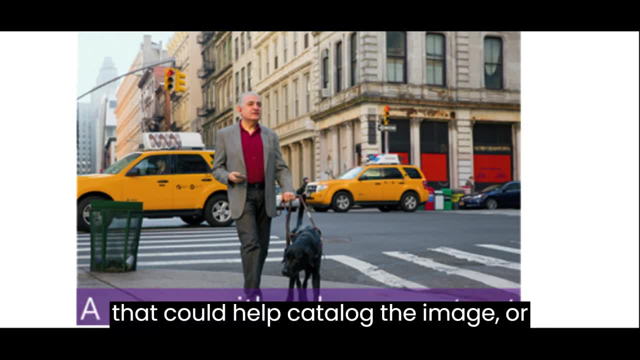 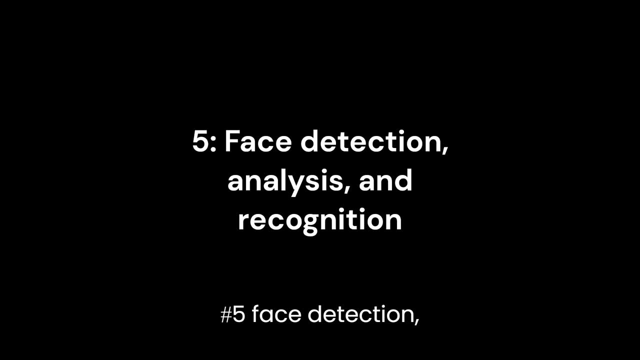 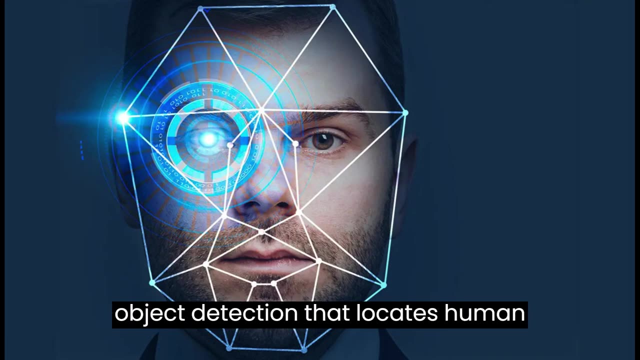 from images, including tags that could help catalog the image or even descriptive captions that summarize the scene shown in the image. Number 5, Face Detection: Analysis and Recognition. Face detection is a specialized form of object detection that locates human faces in an image.